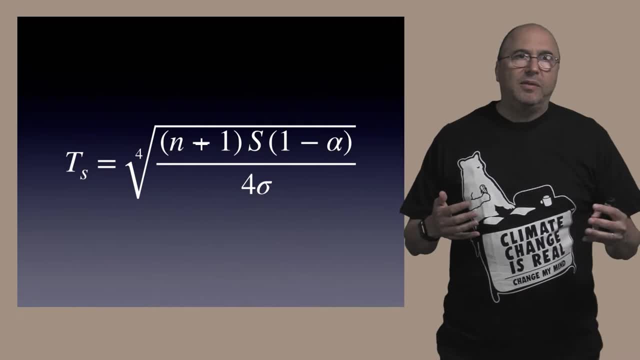 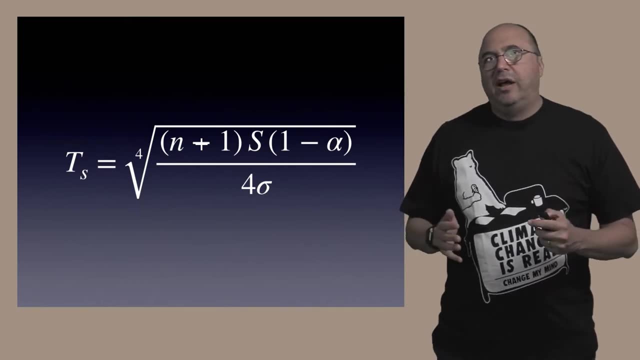 chapter. we're going to dive deep into this question Now. let's begin in this video by describing what our atmosphere is made of. Now, as you probably learned in high school, approximately 78% of the dry atmosphere- I'm excluding water vapor here- is made up of 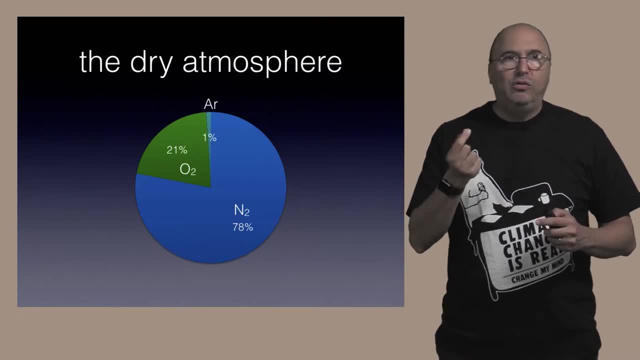 diatomic nitrogen or N2.. These are two nitrogen atoms bonded together. About 21% is diatomic oxygen or O2, which is two oxygen atoms bonded together. This is the part of the atmosphere that we need to breathe to survive. Argon atoms make up approximately 1% of our atmosphere. 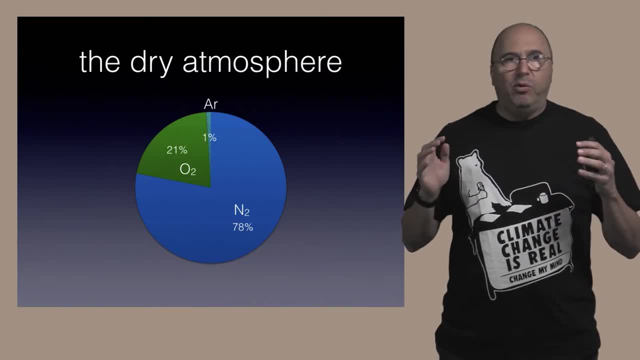 Now, none of these three constituents, which together make up more than 99% of the dry atmosphere, absorbs infrared photons, So they are not greenhouse gases and they don't warm the surface of the planet. The next question we're going to look at is how much of the atmosphere is made up of. diatomic oxygen or O2,, which is two oxygen atoms bonded together. This is the part of the atmosphere that we need to breathe to survive. Argon atoms make up approximately 1% of our atmosphere, and this is the part of the atmosphere that we need to breathe to survive. This is: 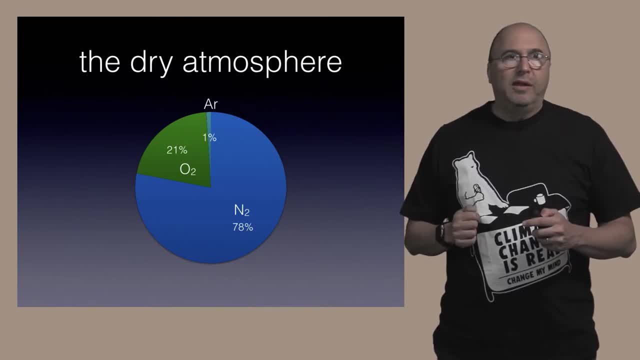 aidoids, the،. these are mostly natural biom qual files and I've covered about 100 of all the different elements in it, but it's aiently 20% because the structure of the diatomic nitrogen atoms is made up of this. The second biggest component to the 5-do is water vapor or H2O. I didn't include it. 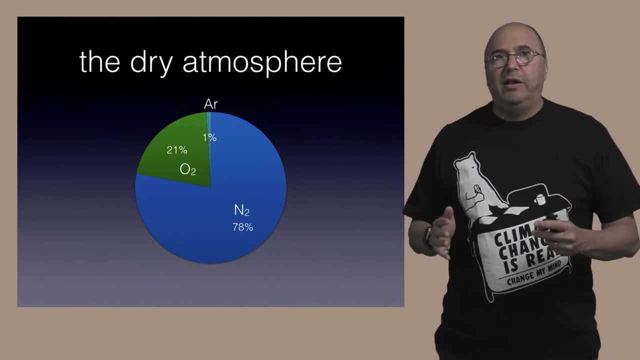 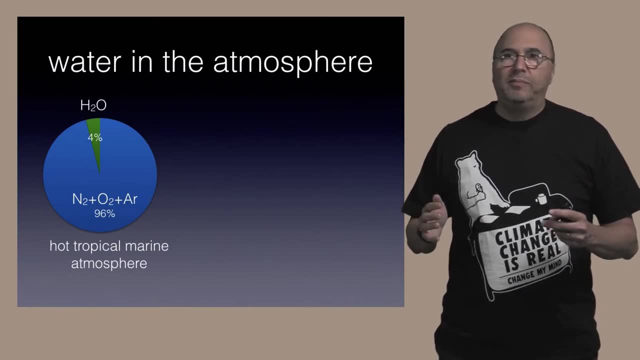 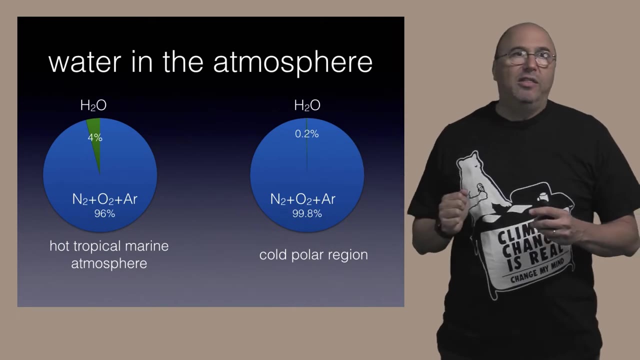 in the plot because it's composition varies greatly from place-to-place. In the warm tropics, water vapor can make up around 4% of the atmosphere. In the cold polar regions, water vapor may only be only 0.2%, and you can barely see it on this pie chart. 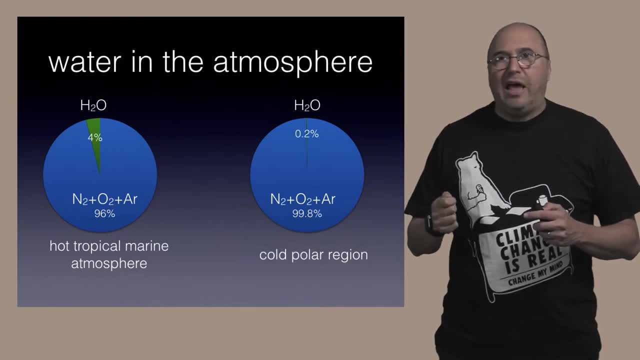 Now during hot winter. in winter, water vapor is the most abundant and the most important greenhouse gas in the atmosphere And you can notice that in the weather Wonderland, our atmosphere. Its main source is evaporation from the surface, mainly the oceans, and it is 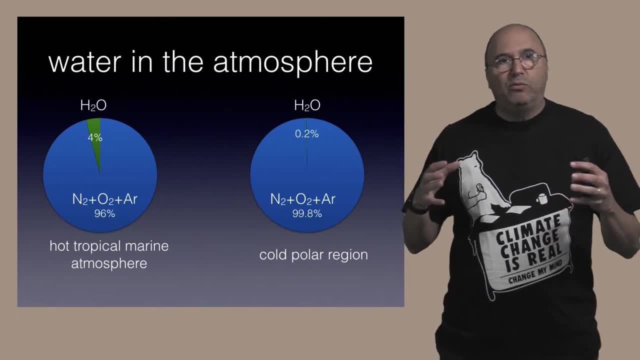 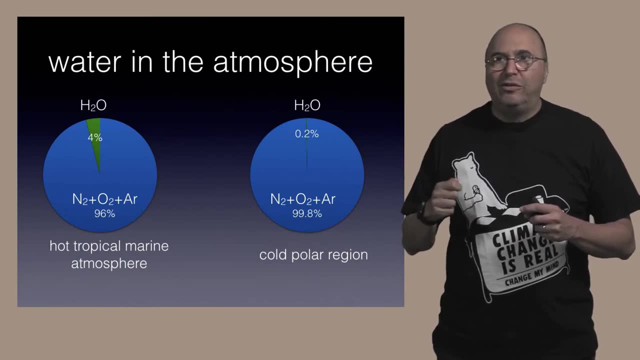 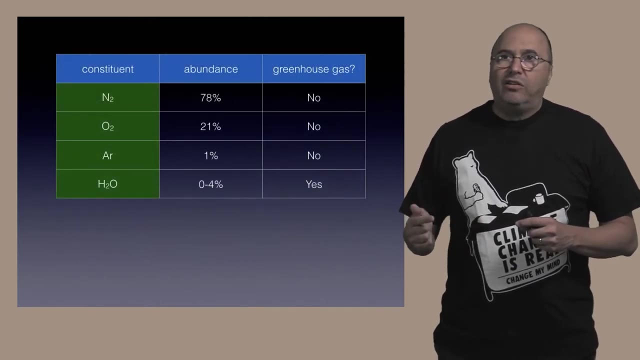 removed from the atmosphere. when water in the atmosphere forms raindrops and these fall onto the surface, Emissions of water vapor from human activities contribute essentially nothing to the atmospheric abundance. So, taken together, nitrogen, oxygen, argon and water vapor make up more than. 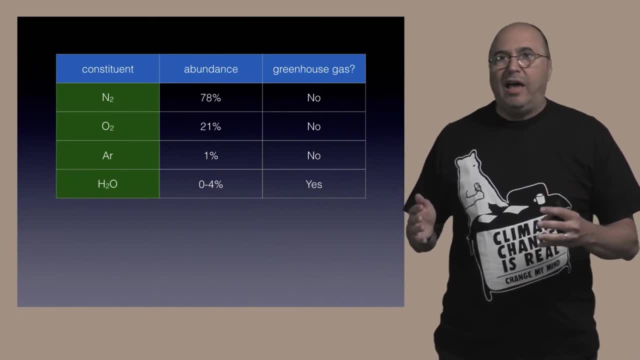 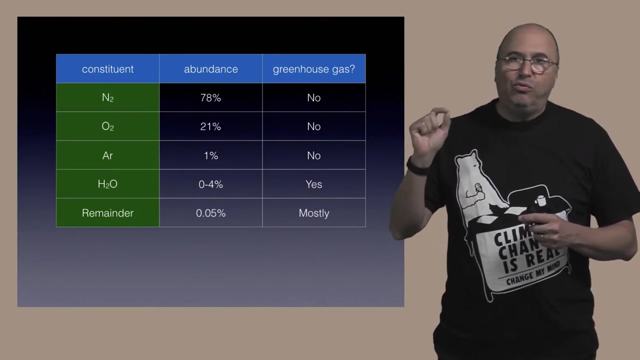 99.95% of the atmosphere. Now you might think that the remaining 0.05% play no important role, because it seems like such a small amount, but you would be wrong. This last smidgen of the atmosphere is actually crucial for life on the planet. So before we talk more about what makes 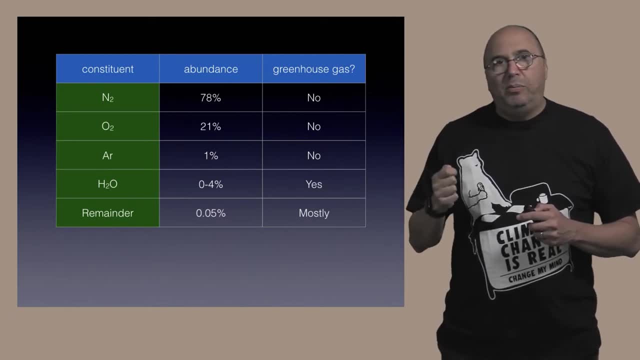 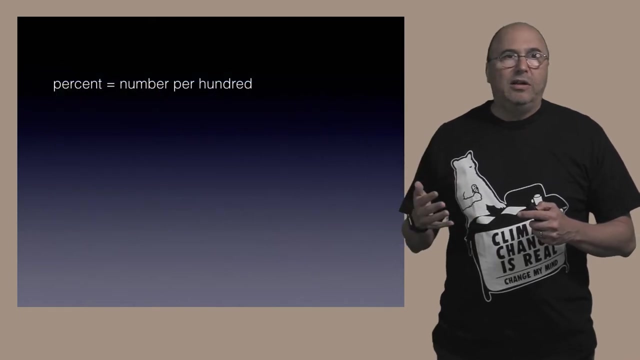 up this last smidgen. let's change units. 0.05% is an awkwardly small number, so scientists typically express the concentration of trace gases in a more convenient unit: we call parts per million. Now, to think about parts per million, let's start by understanding percent. So 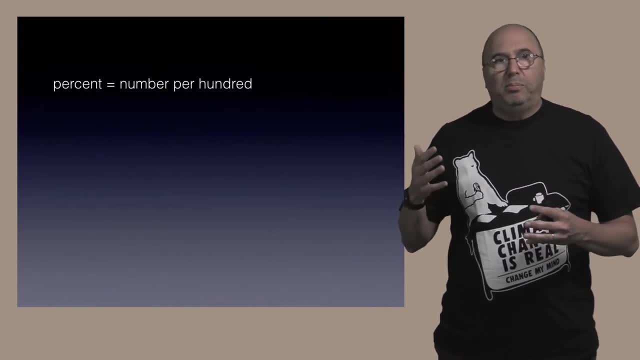 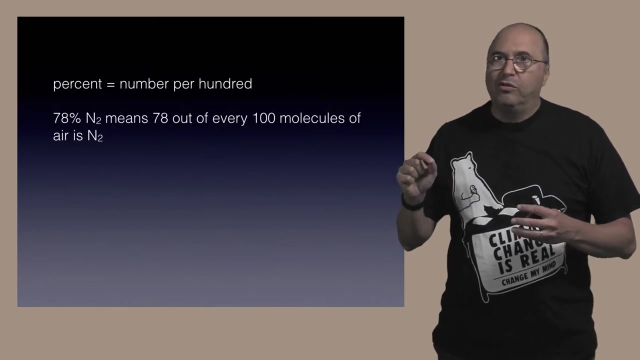 the word percent comes from the marriage of the words per and cent, literally meaning out of a hundred. Thus, air is approximately 78% nitrogen, which means that 78 out of every 100 molecules of air are molecules of nitrogen. A concentration expressed in parts per million is very similar It. 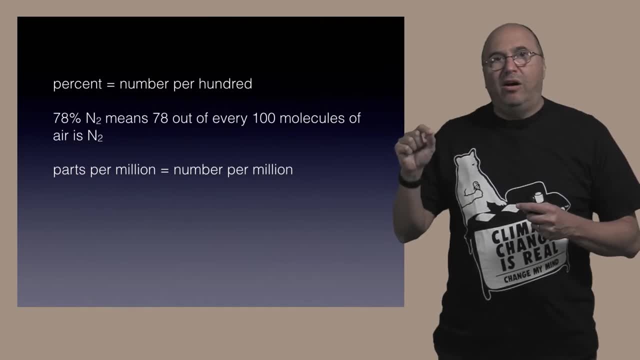 indicates how many molecules out of every million are the gas in question. So, of the 500 parts per million that remain, most are carbon dioxide. At the time that this video is made, in the summer of 2019, the abundance of CO2, carbon dioxide- in our atmosphere was 410 parts per million. This means that each our atmosphere will carry around 400 parts per million, that is, 810, as times. So China's carbon dioxide, which is clean, will last the entire. 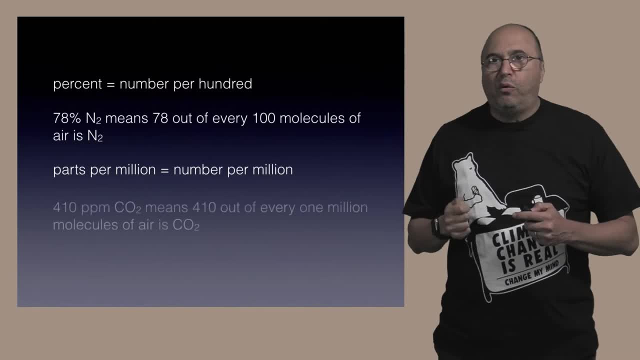 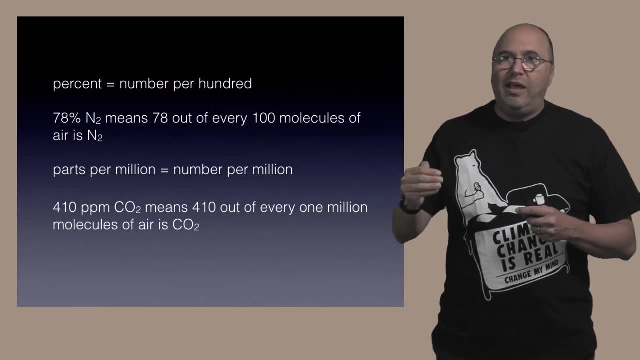 of co2- carbon dioxide in our atmosphere- was 410 parts per million. this means that out of every million molecules in the atmosphere, 410 of them are carbon dioxide. now, carbon dioxide is the most important greenhouse gas for climate change and it's the second most important greenhouse gas. 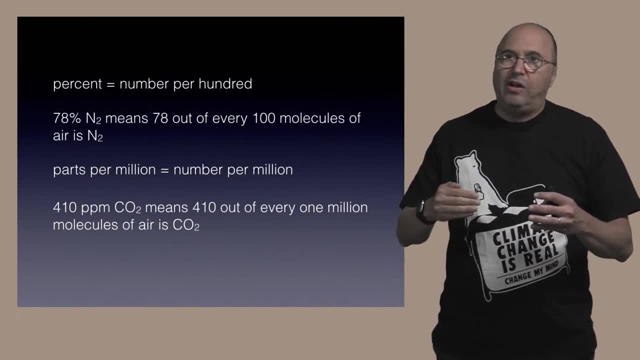 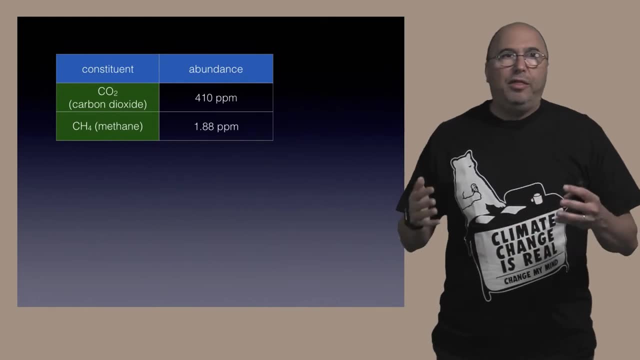 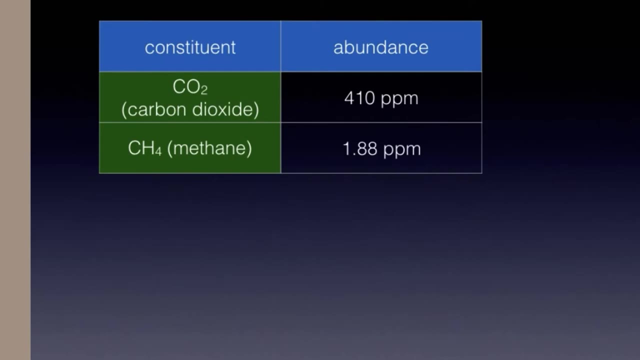 behind water vapor, and we'll talk more about this in this chapter and in chapter six. now, after carbon dioxide, the next most important gas in our atmosphere is methane, or ch4. in 2019, it has an atmospheric abundance of about 1.88 parts per million. despite its small abundance, 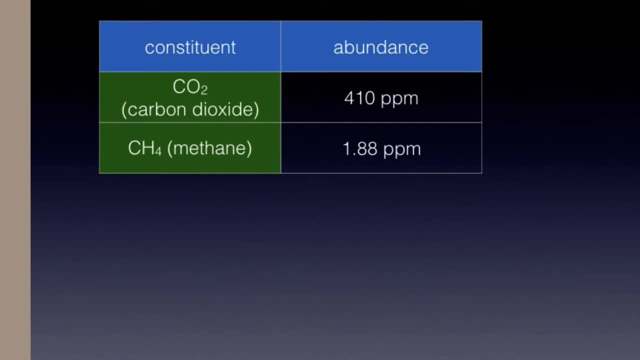 methane is also a key player in our climate system. another important greenhouse gas in our atmosphere is nitrous oxide, or n2o, which is present in today's atmosphere at concentrations of about zero percent of carbon dioxide- 0.32 parts per million. Ozone is another greenhouse gas. 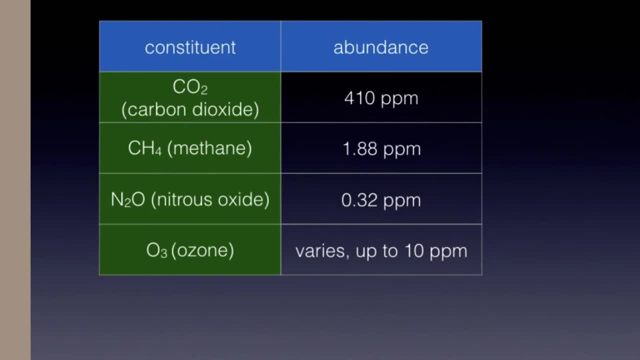 Its chemical formula is O3, so it's a molecule made up of three oxygen atoms. This is different from the form most of the oxygen our atmosphere takes, which is in the form of O2.. The abundance of ozone varies widely across the atmosphere. 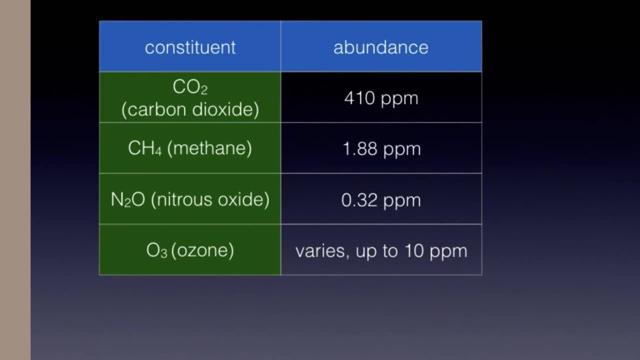 In the stratospheric ozone layer. the abundance can reach 10 parts per million. Now, ozone is not just a greenhouse gas. It's also absolutely necessary for life on our planet, because it absorbs high energy ultraviolet photons emitted by the sun before they reach the Earth's surface. 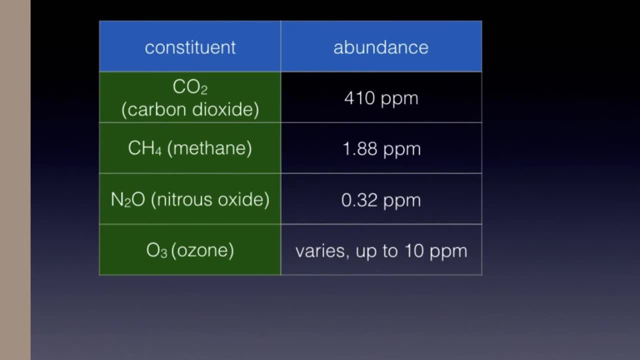 These UV photons are what cause you to tan and they also carry enough energy. they can seriously damage living tissue, leading to diseases such as skin cancer in humans. A final group of greenhouse gases are known as halocarbons, which are synthetic, industrial 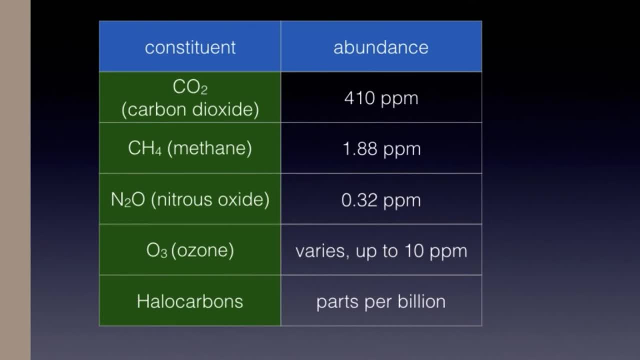 chemicals. These chemicals are used in air conditioners and refrigerators and in various industrial applications. Structurally, they're molecules containing carbon and halogens, hence the name halocarbons. Halogens include chlorine, fluorine and bromine. 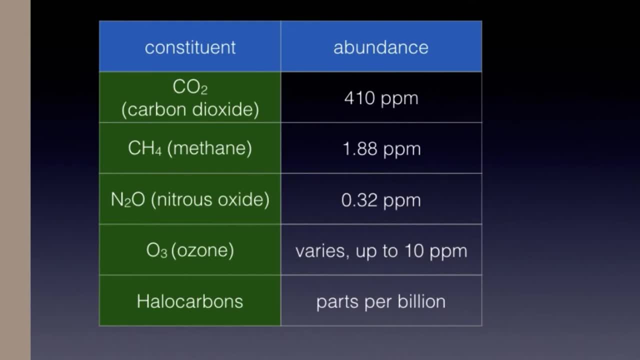 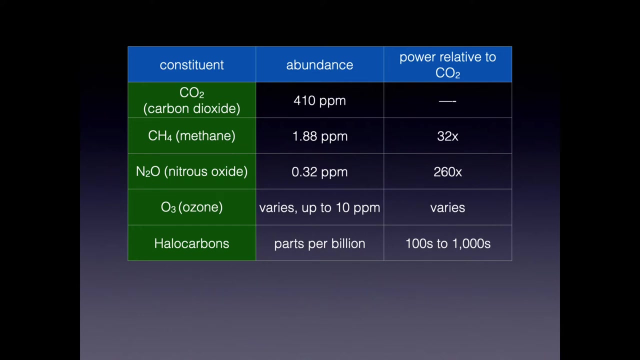 Together. halocarbons are present in today's atmosphere at a concentration of just a few parts per billion, meaning that just a few molecules out of every billion molecules of air are halocarbons. Now, these greenhouse gases are not equal in their ability to warm the planet. 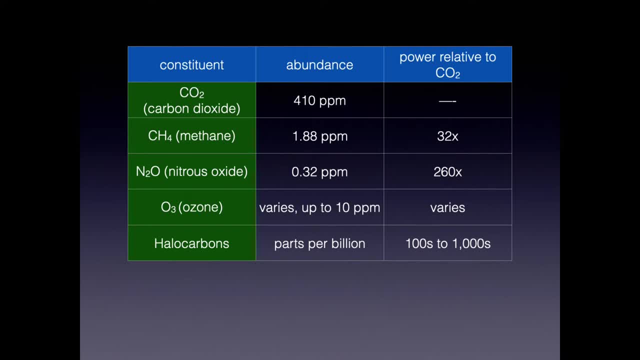 The third column shows the per-molecule warming due to each one relative to carbon dioxide. A molecule of methane is roughly 32 times more powerful of a greenhouse gas than a molecule of carbon dioxide. So while methane has a much lower abundance in the atmosphere, it is strong enough on. 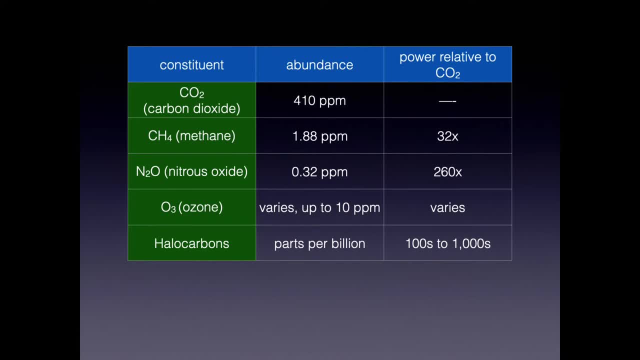 a per-molecule basis to still make an important contribution to the greenhouse effect. The most powerful greenhouse gas on a per-molecule basis are the halocarbons. Each halocarbon traps as much heat as hundreds or thousands of carbon dioxide molecules. 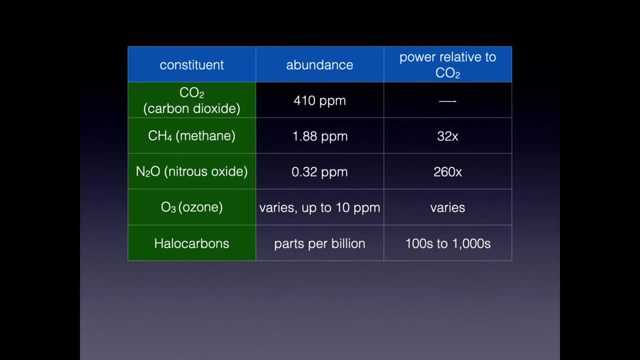 So, despite being about one ten-thousandth as abundant as carbon dioxide, these halocarbons nevertheless make an important contribution to the greenhouse effect. And never forget that the three most abundant gases in our atmosphere- diatomic nitrogen, diatomic oxygen and argon